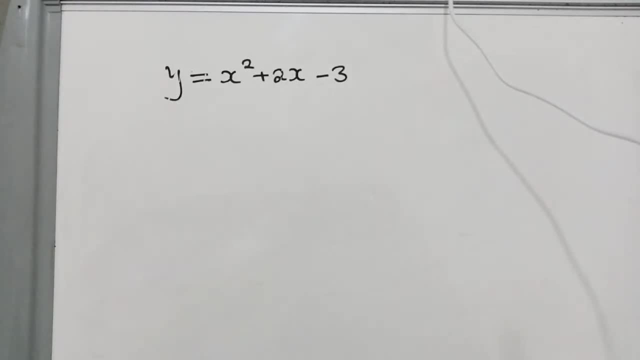 So join, kindly join. Let's graph this. Don't forget to like my video. Hello, how are you? Thanks to know that you have joined our broadcast, So we're going to discuss on how to graph B-trace. Good evening, how are you All right? so if you've just joined, 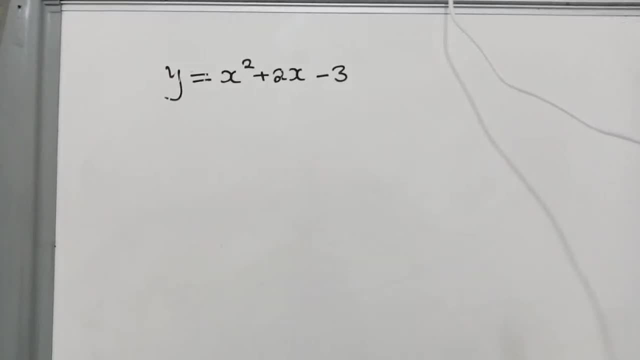 don't forget to like my video and kindly share so that you can have a big audience. All right, so let's start. How do we graph this one? So, on how to graph this one, the first thing will be to find what we call y-intercept, and 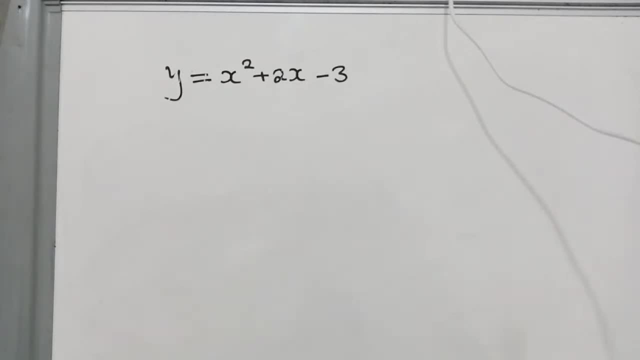 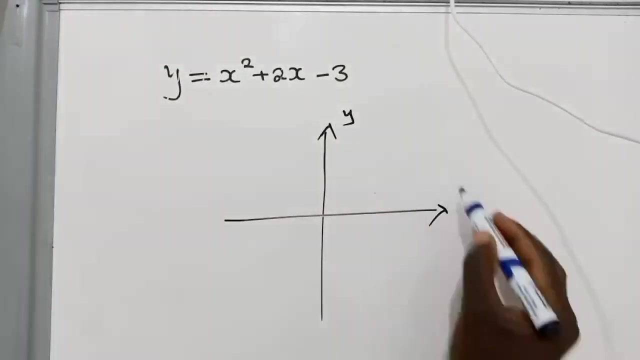 x-intercept. So these are the first two things. So how do we find the y-intercept? So first let me explain what I'm talking about. First of all, let me explain what I'm talking about. So you have a Cartesian plane like this: This is y-axis and this is x-axis. Okay, 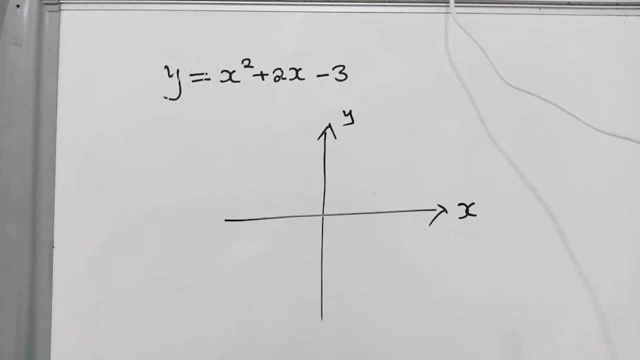 so when graphing, you basically need to know where this graph is cutting: the x-axis, this x-axis and also the y-axis. So for the x-axis, we call it x-intercept. So the things that we need to know are the y-intercept. We have a graph that's called the x-axis and this is y-intercept. 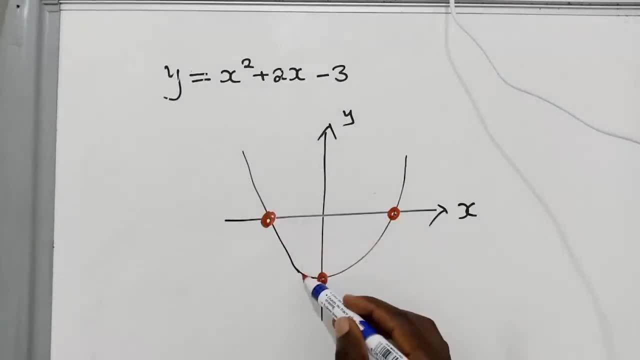 So what we need to know is that when you're looking at the graph, this is y-intercept. if you look at the graph, it's a little bit bad, but all the same. So you need to find here, here, here and the turning point. So let's say the turning point is somewhere here. 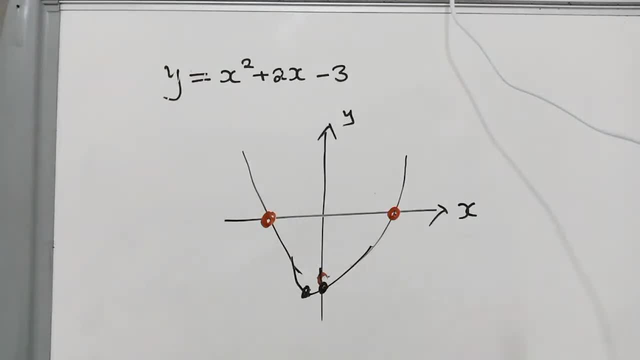 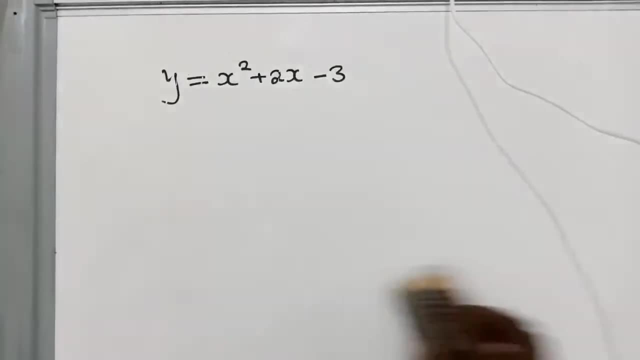 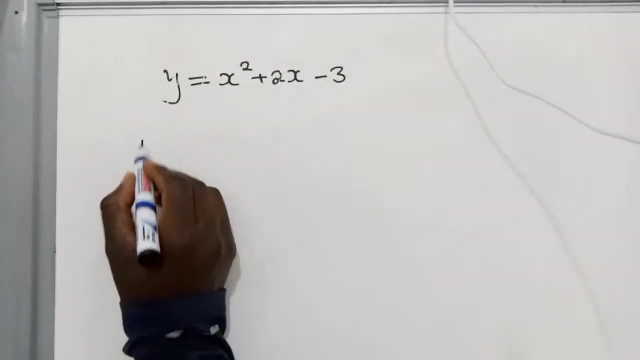 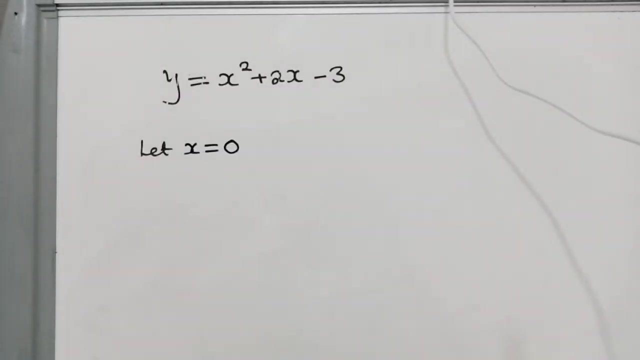 This is the turning point and this is the y-intercept, where it's cutting the y-axis. So now let's find where the graph is passing on the y-axis. So we'll say: let x be equal to 0.. So where this graph will be cutting the y-axis, the x-axis will be 0.. 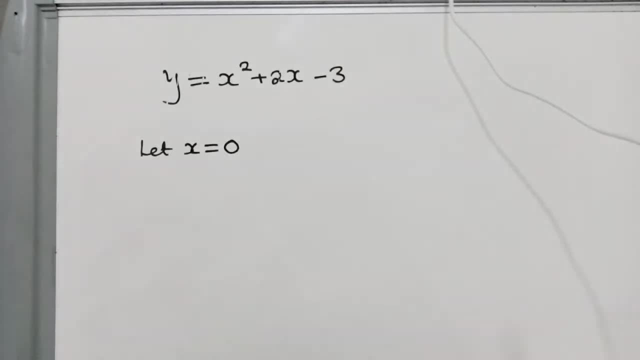 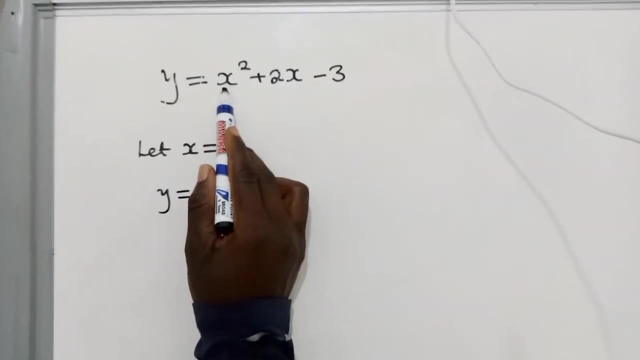 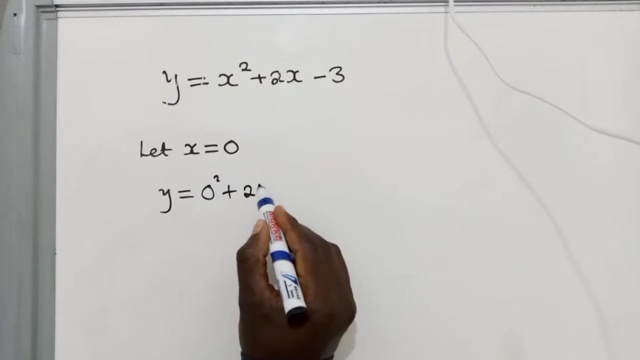 So always remember to put the x-axis as 0. And then you say y is equal to where there is x. we put 0. So it would be 0 plus 2, here 0 squared plus 2, here 0 minus 3.. 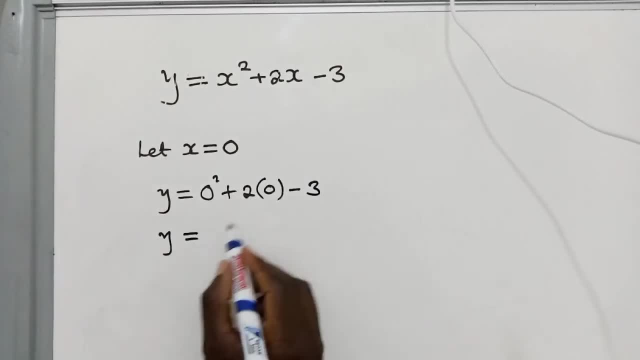 So once you do so, when you solve nicely, you find that your y-axis will be equal. So we'll say y is equal to negative 3.. This is 0 and this is 0, so we'll just say: remain with the negative 3.. 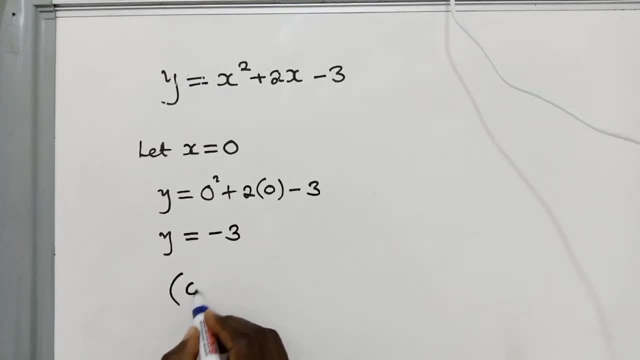 So we have a set of coordinates: 0, negative 3. This 0, we know that this is x-axis, it's 0. And y-axis is negative 3.. So this is a set of the coordinates we need to have. 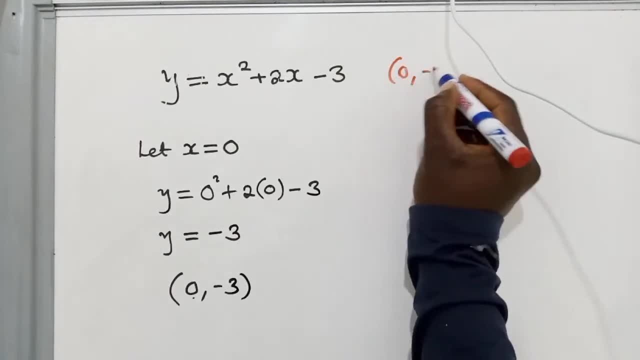 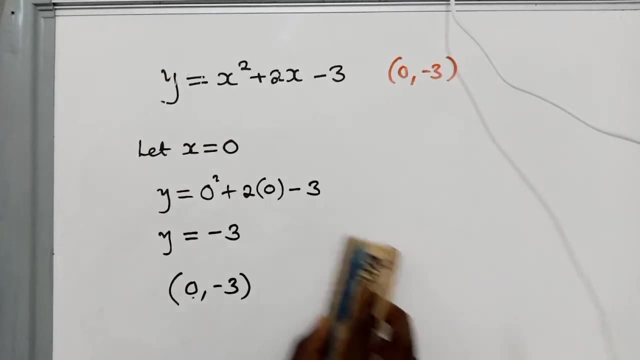 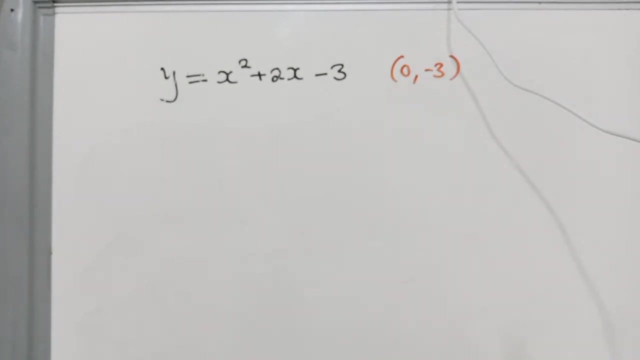 So we'll keep them, we'll put them here. So we have that. The next thing now will be to find what we call x-intercept. So we need to also find where it's passing at x or where it's cutting the x-axis. 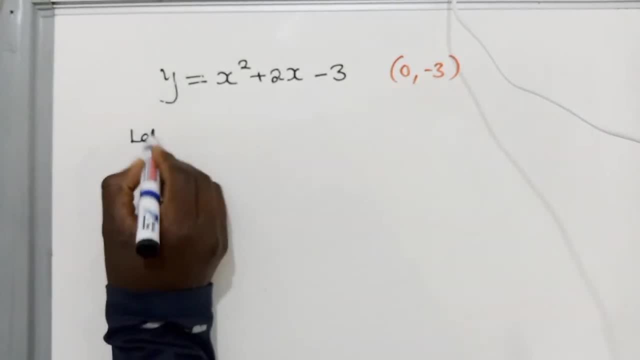 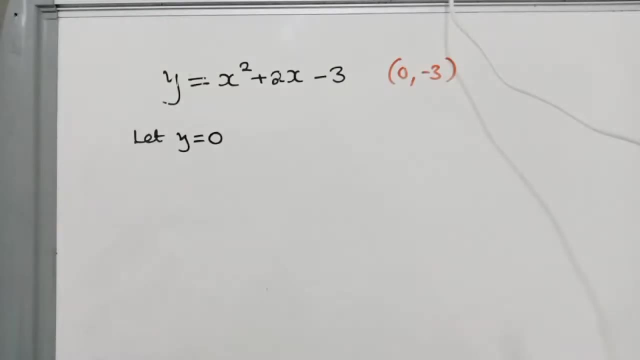 So now we'll change. we'll say let y is equal to 0. To find this, we set let x be equal to 0. So now we'll say let x be equal to 0. y is equal to zero. so meaning on or in this function, we'll put zero where y is. so we're. 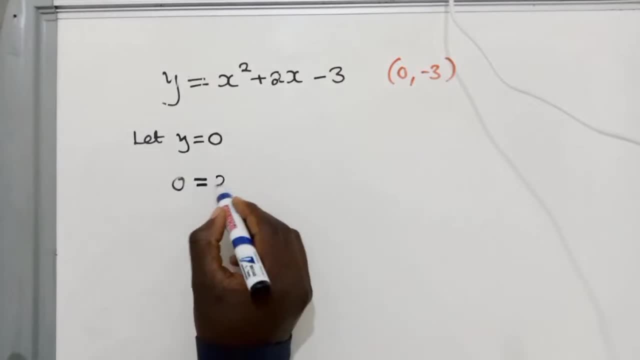 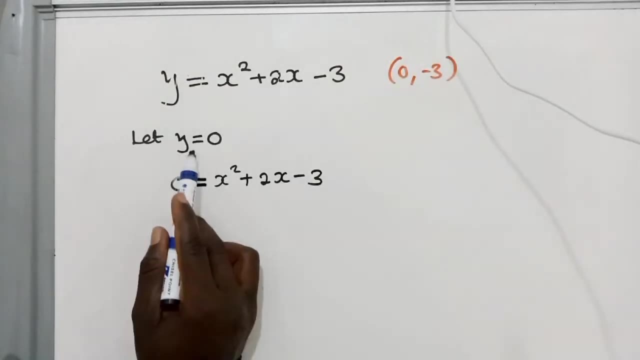 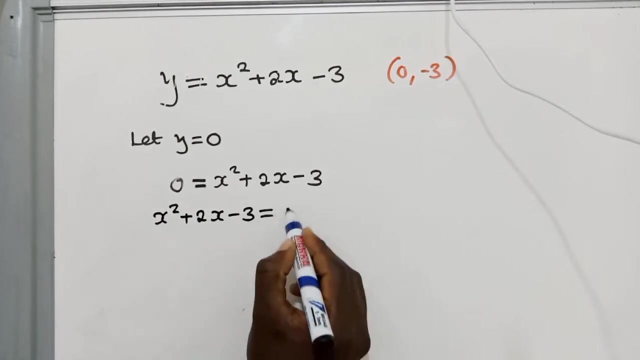 going to say: zero is equal to x squared plus 2x minus 3. so this y is equal to zero, is the one i've put here. so you can see there is zero here. so if you're able to see nicely following what is going on here, you find that this is simply the quadratic equation, solving the quadratic. 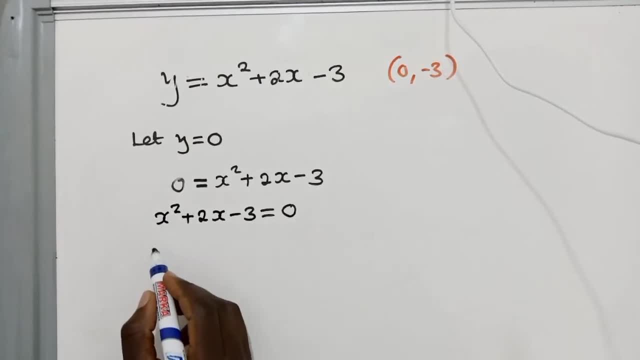 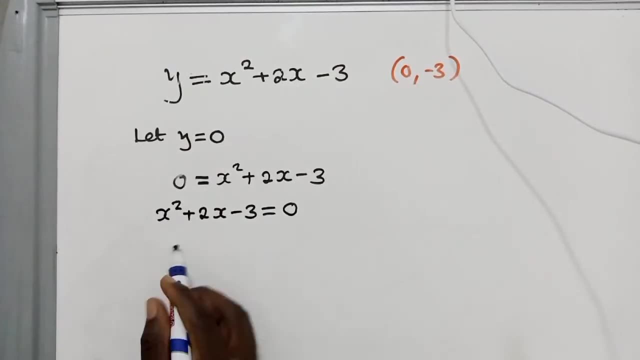 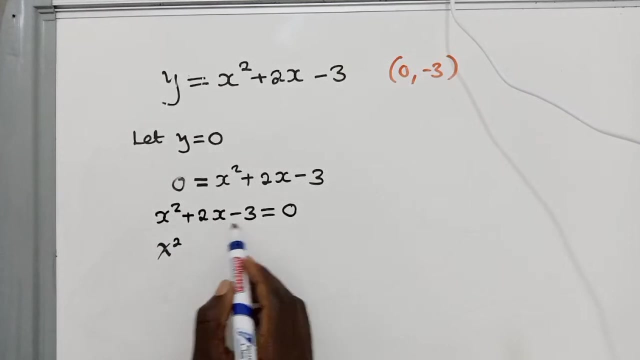 equation. so how do you solve the quadratic equation? if you have an idea of solving the quadratic equation, you simply say you find the, the factors. okay, two numbers such that when you multiply them they give you negative three, and when you add them they give you uh, two, and these numbers are three. 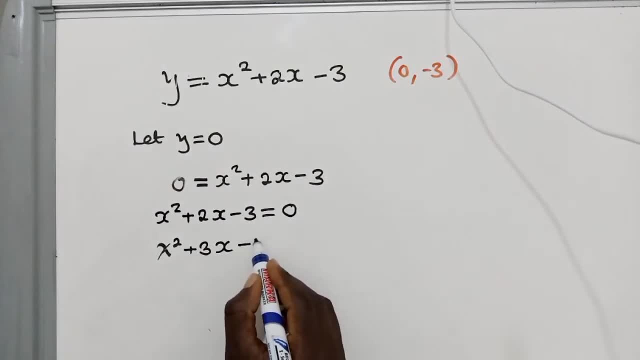 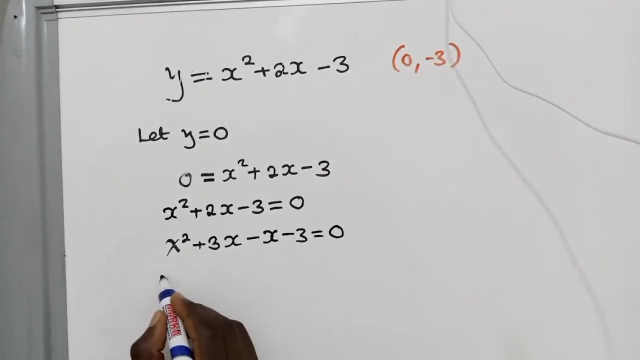 and one. so these numbers are three and one. in case you don't know, on how to solve the quadratic equation, you can check one of my videos where i've explained on how to solve a quadratic equation. i think i'll put you. i'll put the link in the description. so now, when we solve here, you have something like this: 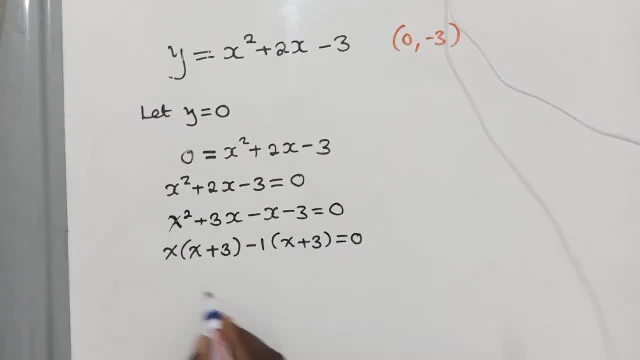 so this is just this quadratic equation. we're solving the quadratic equation whereby we have something like this here, so if you need me to explain here, kindly let me know so that i can explain. maybe you're very behind, but if you're okay, that is. uh, that is a plus to me. 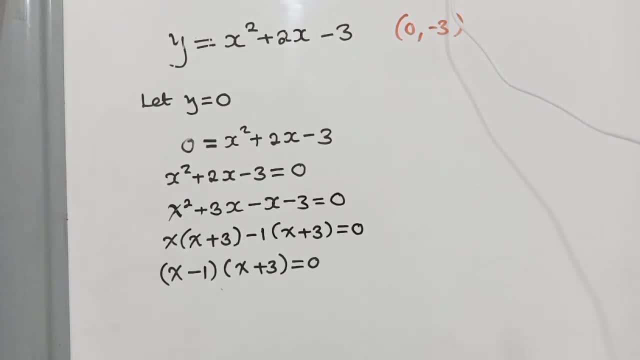 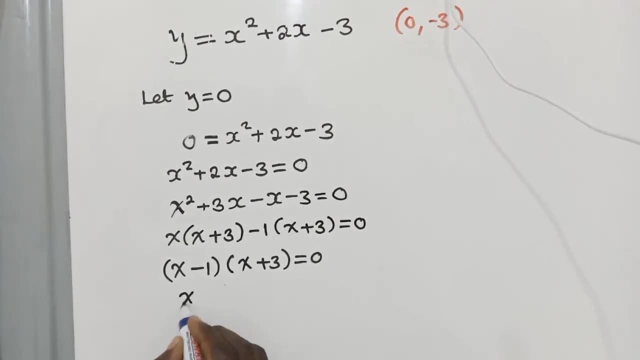 okay, if you're okay, i am. i'm happy if you're okay on how to solve a quadratic equation here. so we're done here. so we can now say x is equal to one or x is equal to negative three. so these are the x values. so now what we're doing here is that we're going to solve the quadratic equation. 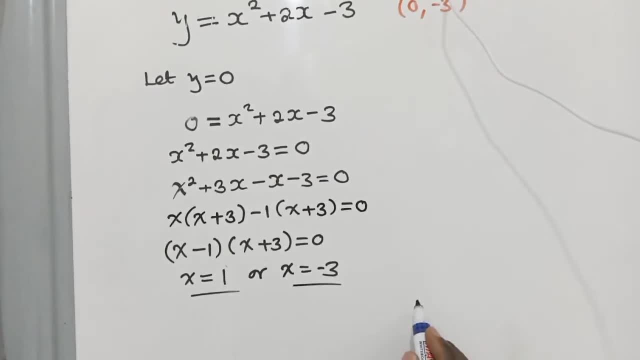 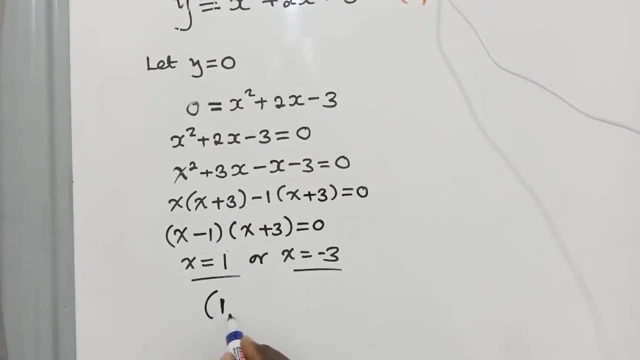 now what we are going to do is to find the coordinates, okay, or to put the coordinates here. so say: x is 1 comma y. we said 0, so y is 0. the other one negative 3 comma 0. this x is negative 3 comma, the y is 0. so you see, we have these coordinates. oh, good evening. uh, glitters, thank. 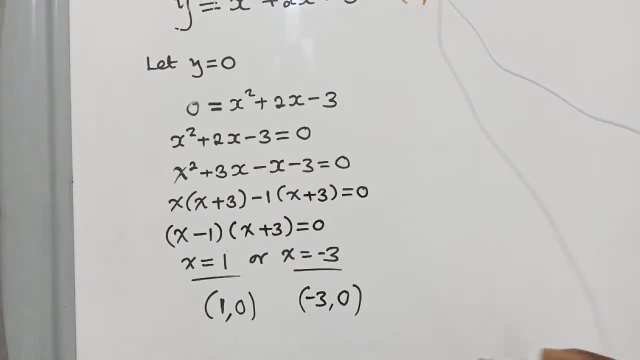 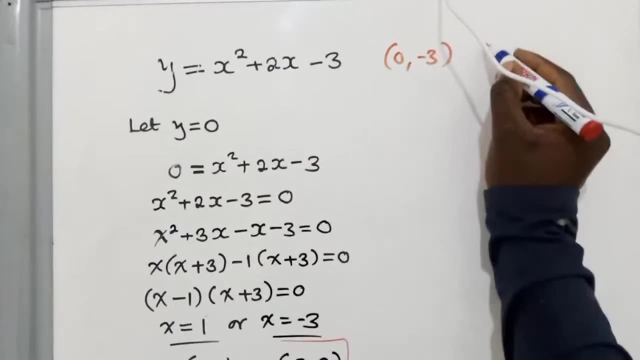 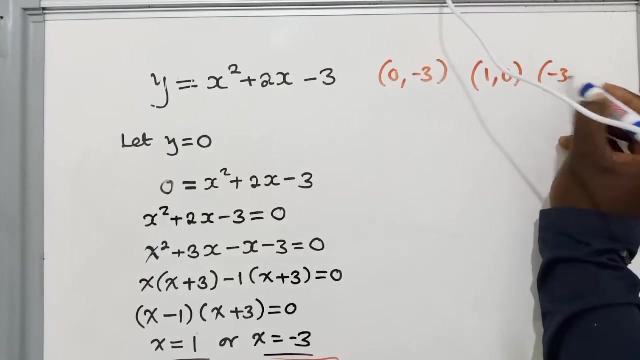 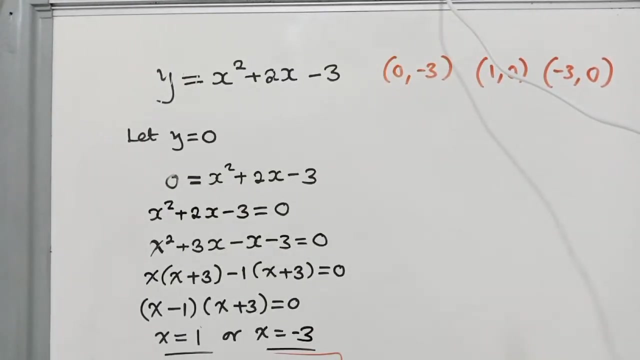 you very much to know that you are. you are watching and following, so now get these coordinates. okay, we'll put them here. we need to use them. we'll put them here. so it was this. and negative 3 comma 0. so these are the coordinates of which now we can graph, but before we graph, 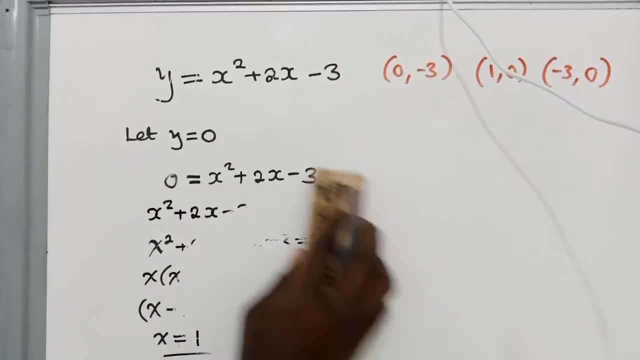 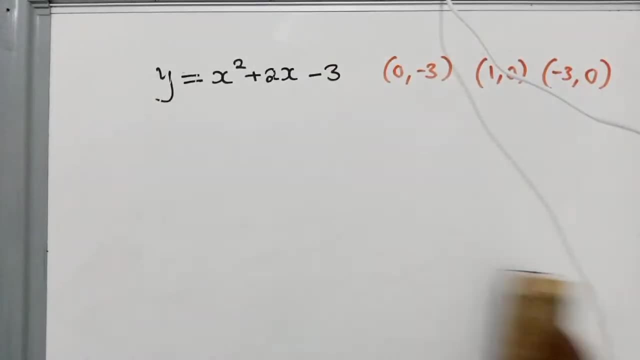 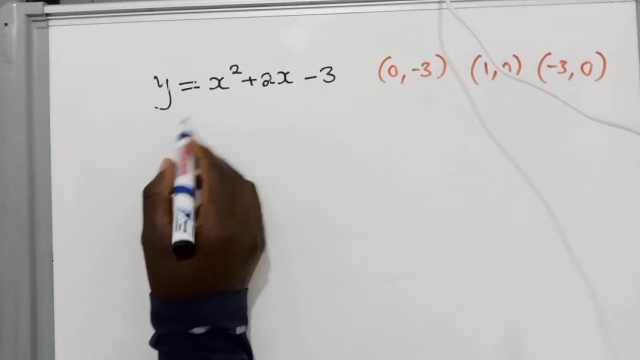 we also need to find the turning point. so how do you find the turning point? how do you find the turning point? so, uh, to find the turning point, there is the formula we use. there are two formulas, so i'll go by this one to find the x value. so this is the formula. 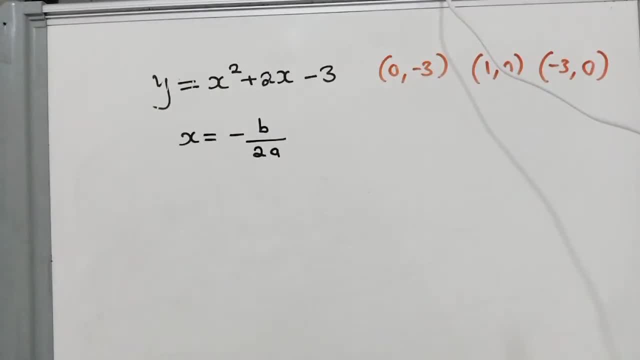 wherever you have been asked to find the turning point, you can use it this formula. thank you very much. uh, good evening since good evening, good evening, all right. so so this is the formula for finding the turning point. you first find the x value whereby you you check what is our b. 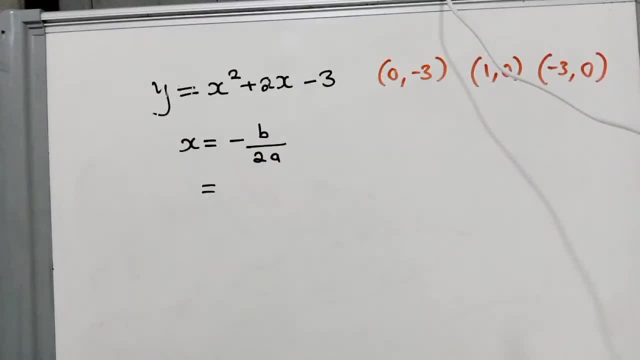 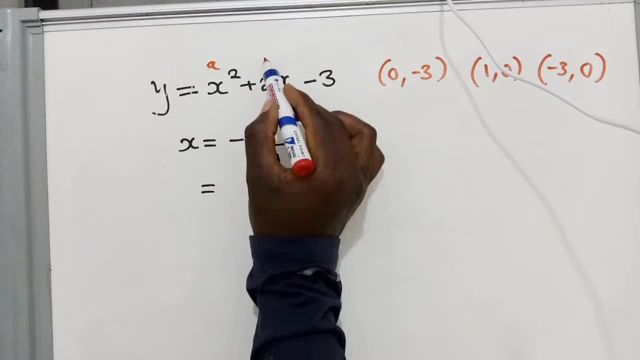 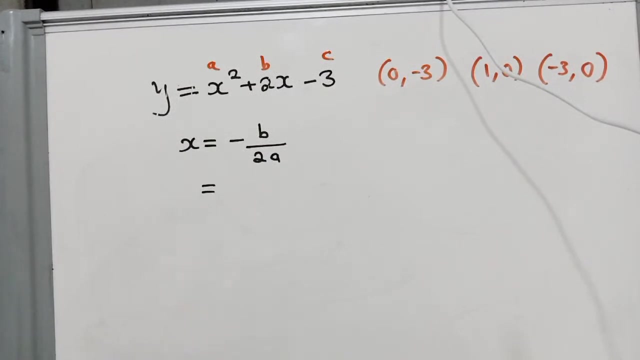 our b is over here. i guess you all know the, the, the standard form of a quadratic function. this is our a, b and the c is here. so for us to find the turning point, we only need a and b. so what is our a? i mean, what is our b? our b is 2 over these two. what is our a is our a is z. 1. there is ahow to calculate the point, to find the turning point three. this will give you the key, so i will show you a solution. we used to find the turning point. there is a h Vietnamese, that is in English. your to find the final zero because you min out a little bit, but you are now. او فاربة. oh who, we are close. so for us to find the turning point, you will only need a and the b. i mean, what is our b? our b is 2 over this two. what is our a, our a, Our a is 1.. 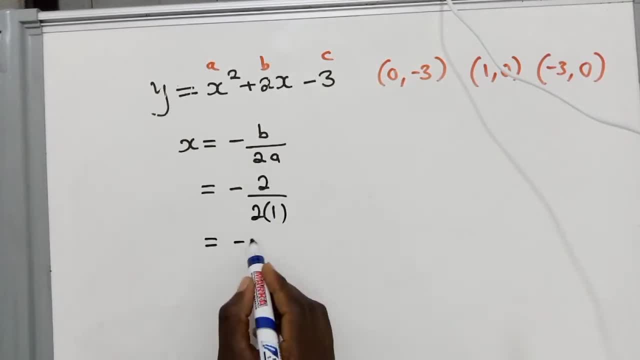 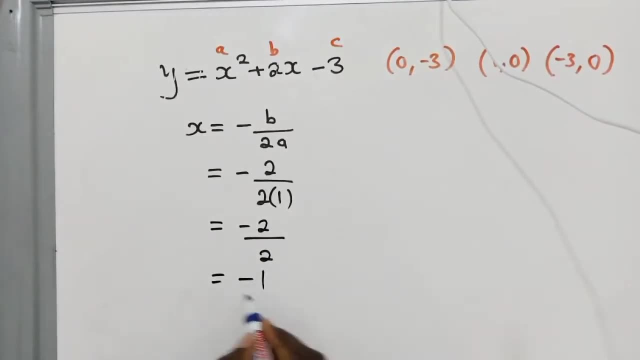 the one here, the coefficient. so you solve, when you solve nicely, you find that, uh, the x value is negative one. this is x value is negative one. okay, because if you say two in two negative, two is just negative one. so now get this x value, put it in this. remember, we are looking for the 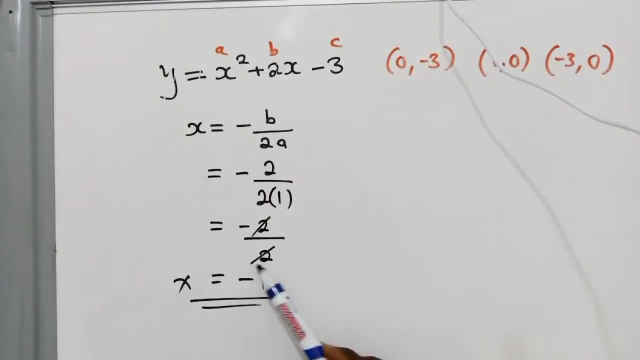 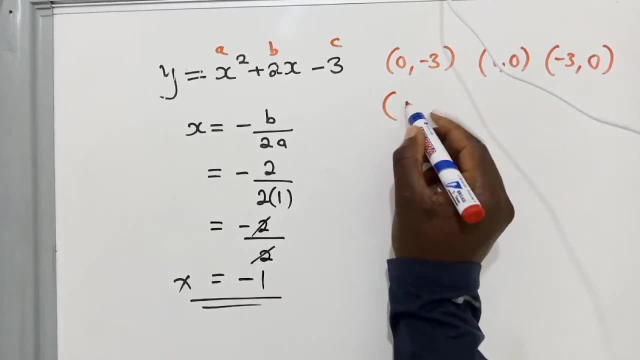 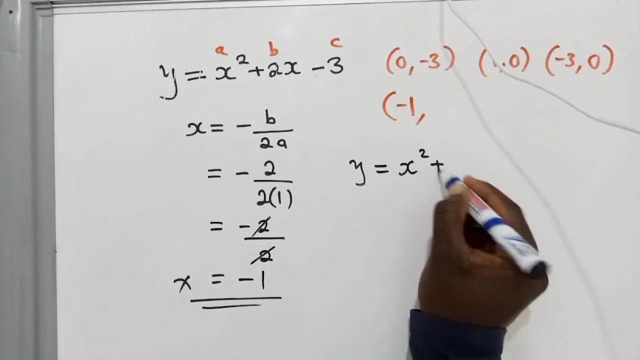 coordinates of the turning point. okay, so now we already have the x value. so we can even write like this, if you want. we can say: for the turning point, x is negative one. what about y? so the y value will just say: y is equal to x squared plus 2, x minus 3, meaning we will get 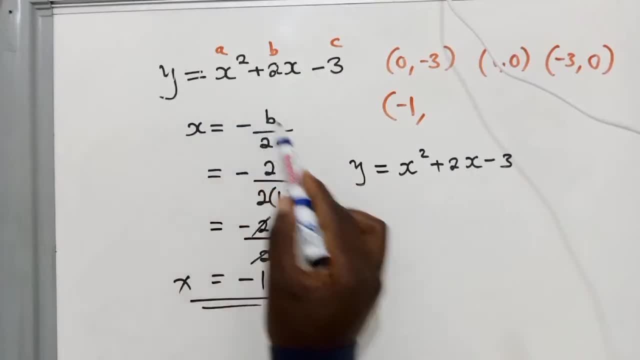 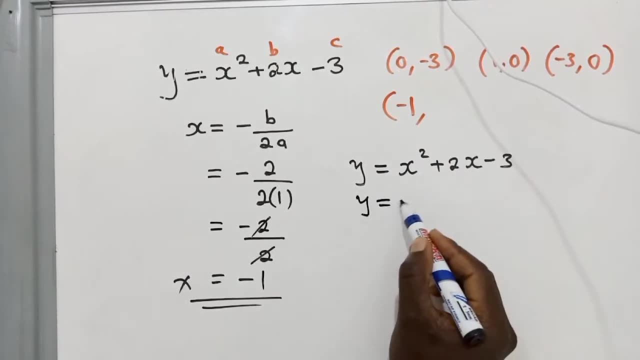 this function. okay, we'll get the function over here and then we get this x value. put it where x is. we're just replacing. so it will look like this: you see i've put negative 1 where x is. i've replaced x with the negative 1. 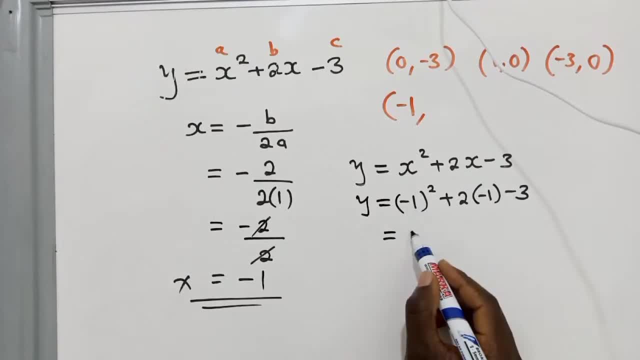 of which, when i say negative 1, squared is just 1. here it will be negative 2, because 2 by negative 1 is negative 2 minus 3, of which, when we work out things nicely here, we'll find that we have. we have something like this, and finally our y value will be equal. 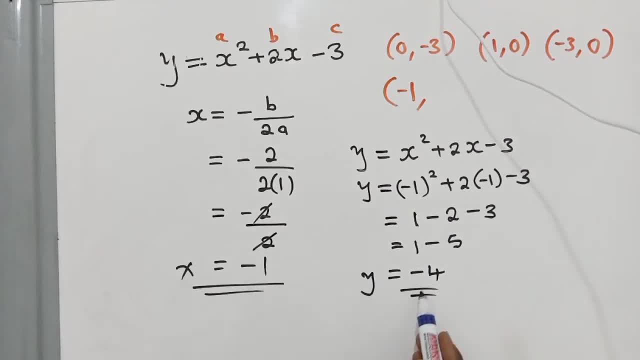 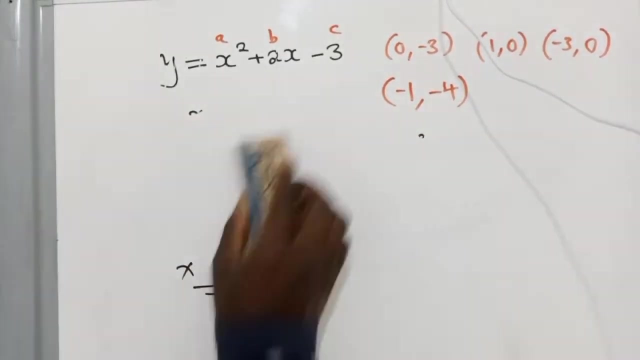 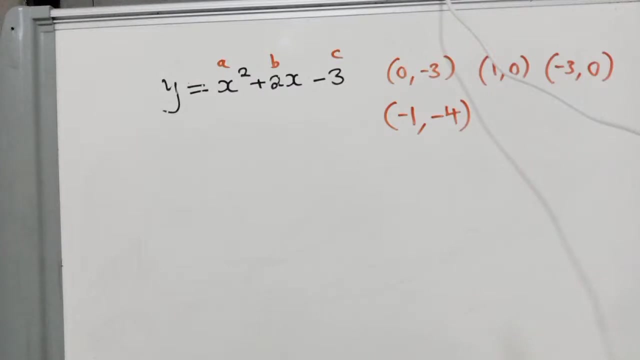 to negative 4. okay, x value, y value. so now we can plug over here. so it will be like this: so we have all this, all the coordinates. in this case, our graphing will be will be fantastic, it will be well done, because we have all the coordinates, all the needed coordinates. so now we can start, we can put our cartesian plane. 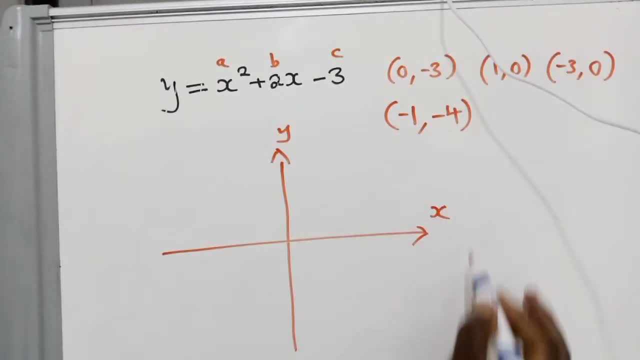 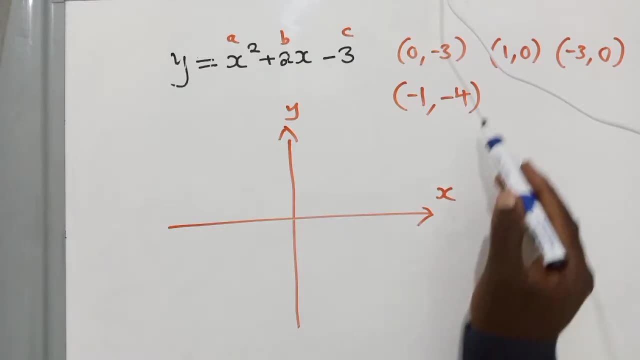 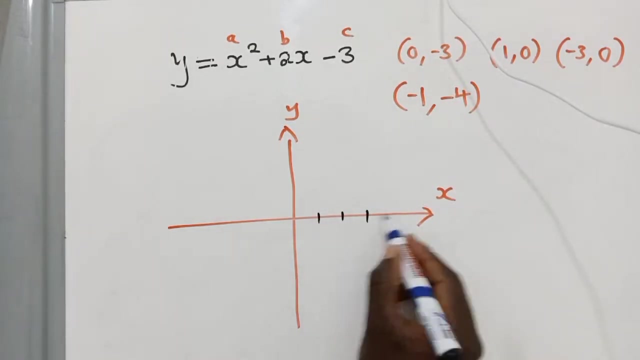 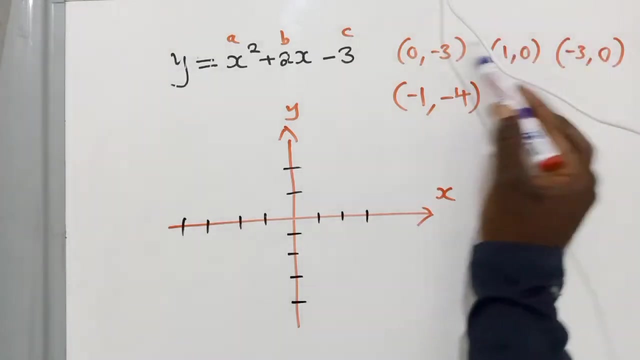 like this: this is y axis and this is x axis, okay, and then we just, uh, we start with, we can start which, we with whichever we want. so this is maybe one, two, three, one, two, three, four. one, two, three, four, one, two. okay, whichever number or whichever range you'd like to, but it should be accommodating these coordinates. so here it's a. 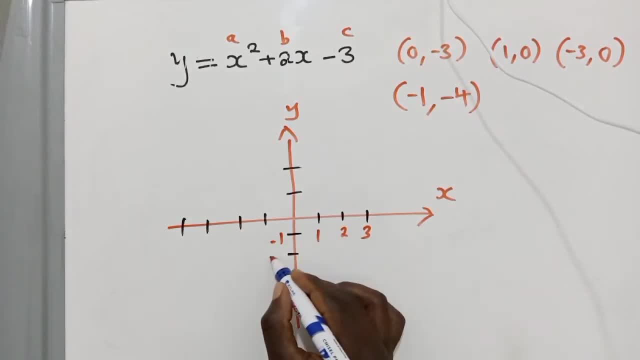 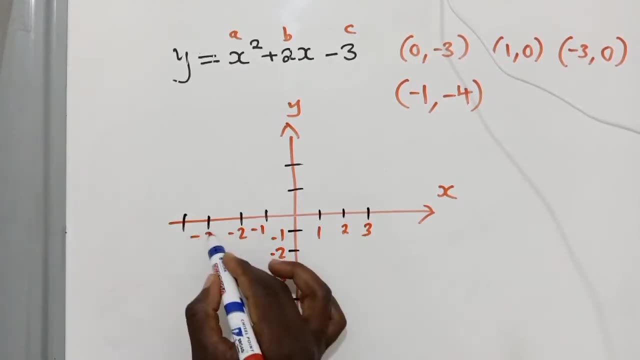 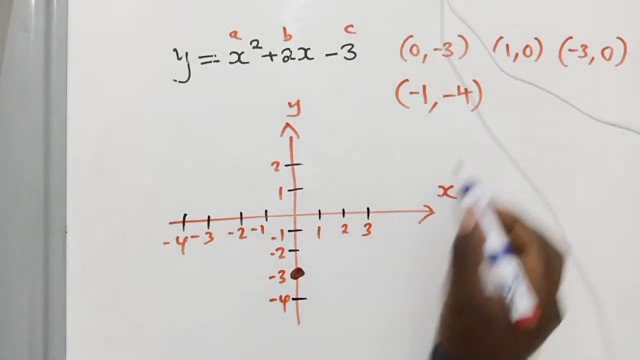 one, two, three here. negative one, negative two and negative three negative four over there. one negative two, negative three, negative four, one, two. so the first there is see zero. comma negative three zero here. comma negative three, it's somewhere here. the next is one comma zero. one comma zero is here. the next is negative three comma zero, it's over.